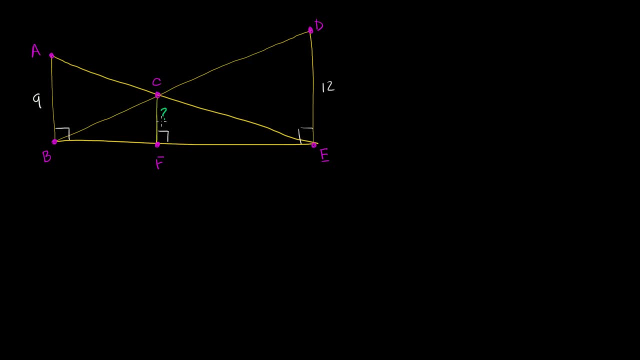 So you have this 90-degree angle in ABE and you have this 90-degree angle in CFE. If we can prove just one other set of corresponding angles is congruent in both, then we've proved that they're similar. And then we can. 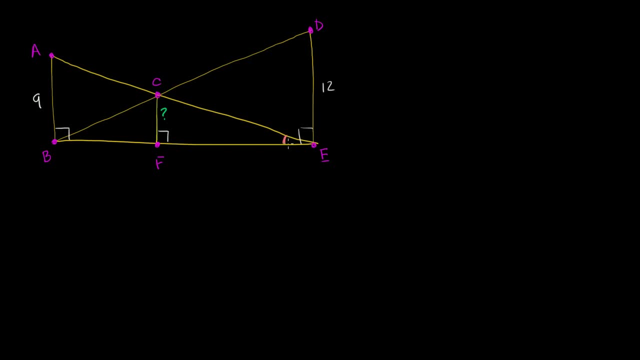 We can either show that. look, they both share this angle right over here. Angle CEF is the same as angle AEB. So we've shown two angles, two corresponding angles in these triangles. This is an angle in both triangles. They are congruent. so the triangles, 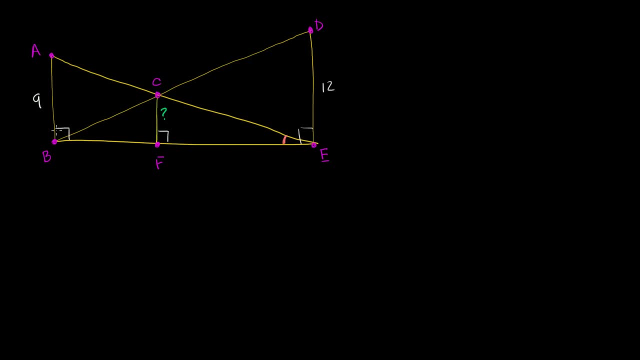 are going to be similar. You could also show that this line is parallel to this line, because obviously these two angles are the same And so these angles will also be the same. So they're definitely similar triangles. So let's just write that down. get that out of the way. 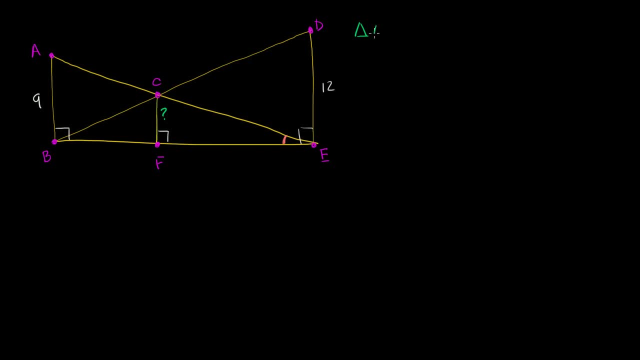 We know that triangle ABE is similar to triangle CFE And you want to make sure you get in the right order. F is where the 90-degree angle is, B is where the 90-degree angle is And then E is where this orange angle is. 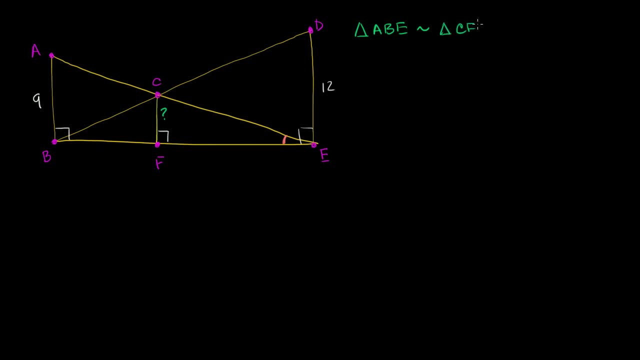 So CFE? It's similar to triangle CFE. Now let's see if we can figure out that same statement going the other way. looking at triangle DEB, Once again, you have a 90-degree angle here. If this is 90, then this is definitely going to be 90 as well. 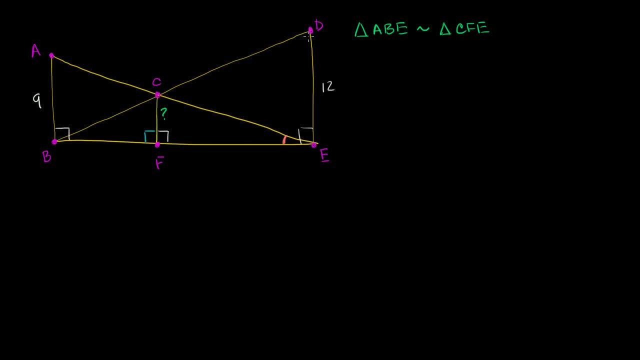 You have a 90-degree angle here at CFB. You have a 90-degree angle at DEF or DEB, however you want to call it. So they have one set of corresponding angles that are congruent, And then you'll also see that they both 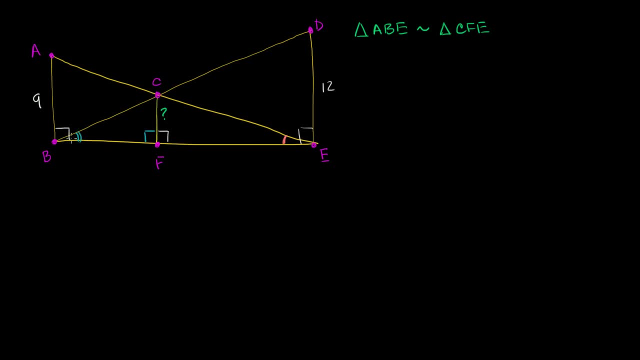 share this angle right over here on the smaller triangle. So I'm now looking at this triangle right over here as opposed to the one on the right, So they both share this angle right over here. DBE Angle. DBE is the same as angle CBF. 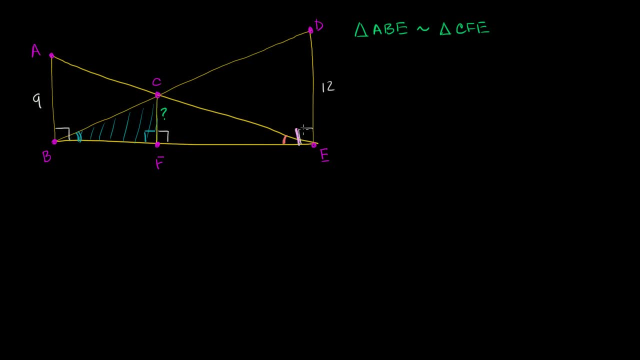 So I've shown you already that we have this angle is congruent to this angle And we have this angle as a part of both. So it's obviously congruent to itself. So we have two angles, two corresponding angles that are congruent to each other. 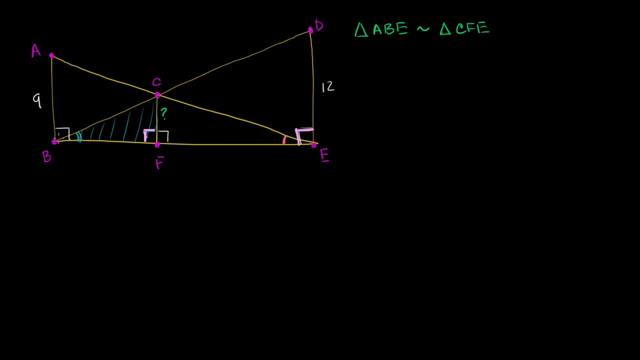 So we know that this larger triangle over here is similar to this smaller triangle over there. So let me write this down. So we also know. let me scroll over to the right a little bit: We also know that triangle DEB is similar to triangle CFB. 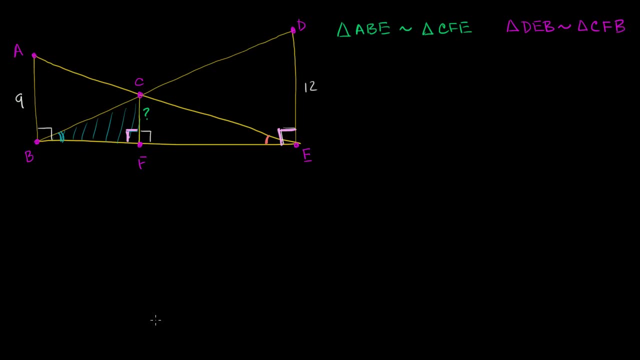 Now, what can we do from here? Well, we know that the ratios of corresponding sides for each of those similar triangles are going to have to be the same, But we only have one side. So in the case of AB and CFB, we've only been given one side. 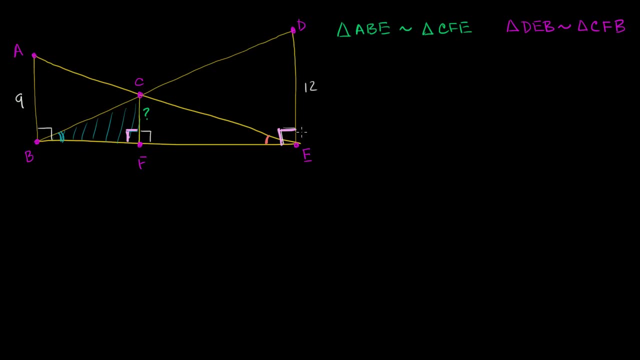 In the case of DEB and CFB, we've only been given one side right over here, So there doesn't seem to be a lot to work with, And this is why this is a slightly more challenging problem. here, Let's just go ahead and see if we can assume one of the sides. 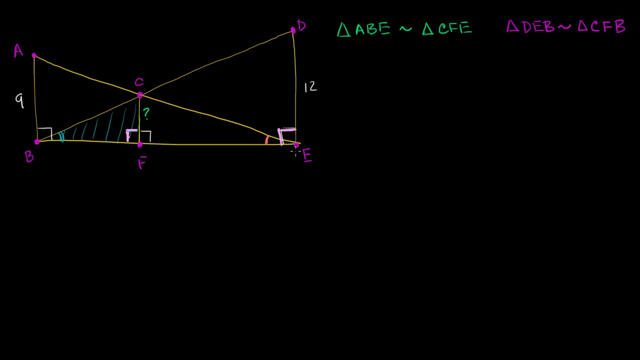 and actually maybe a side that's shared by both of these larger triangles, And then maybe things will work out from there. So let's just assume that this length right over here, let's just assume that BE is equal to y. OK, So let me just write this down. 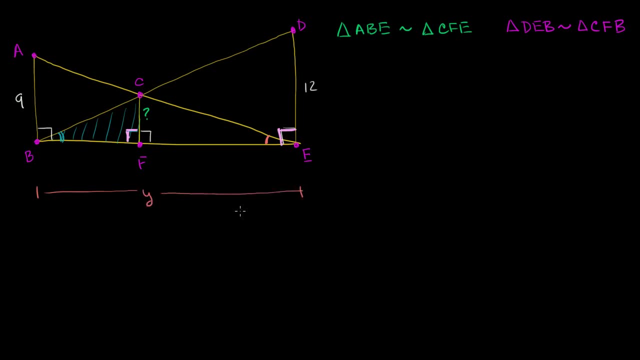 This whole length is going to be equal to y, because this at least gives us something to work with, And y is shared by both ABE and DEB, so that seems useful. And then we're going to have to think about the smaller. 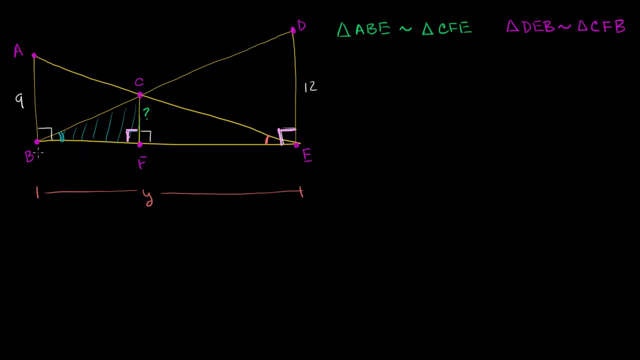 triangles right over there. So maybe we'll call this length, we'll call BFX, Let's call BFX, And then let's call FE. Well, if this is x, then this is y minus x. So we've introduced a bunch of variables here. 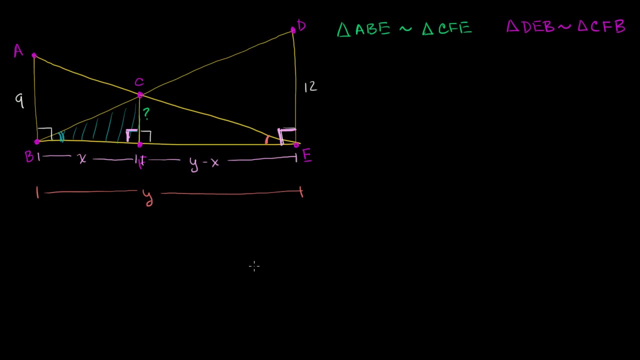 But maybe with all the proportionalities and things, just maybe things will work out or at least we'll have a little bit more sense of where we can go with this actual problem. But now we can start dealing with the similar triangles, For example. so we want to figure out what CF is. 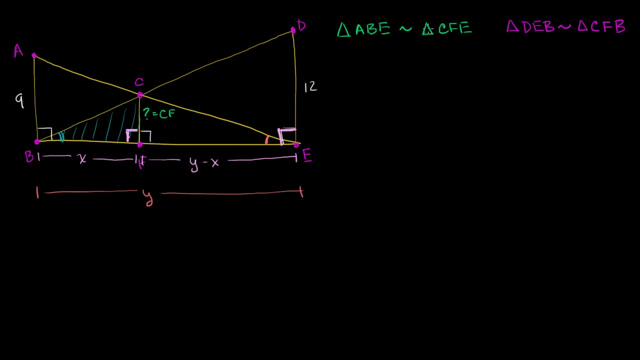 We now know that for these two triangles right here, the ratio of the corresponding sides are going to be constant. So, for example, the ratio between CF and 9, the corresponding sides, the ratio between CF and 9 has got to be equal to the ratio between y minus x. 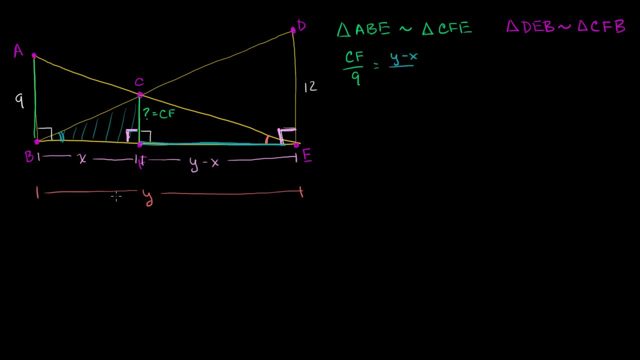 that's that side right there, y minus x, and the corresponding side of the larger triangle. Well, the corresponding side of the larger triangle is this entire length And that entire length right over there is y, So it's equal to y minus x over y. 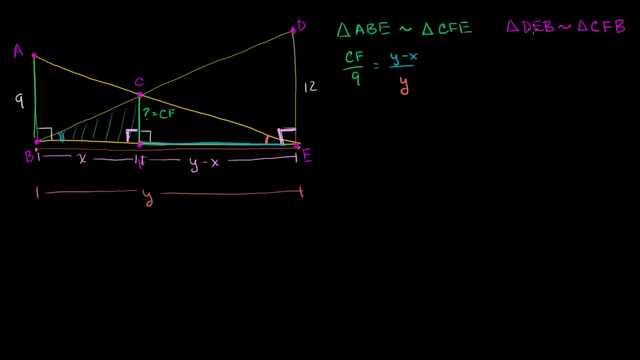 So we could simplify. Let's simplify this a little bit. Well, I'll hold off for a second. Let's see if we can do something similar with this thing on the right. So once again we have CF, its corresponding side on DEB. 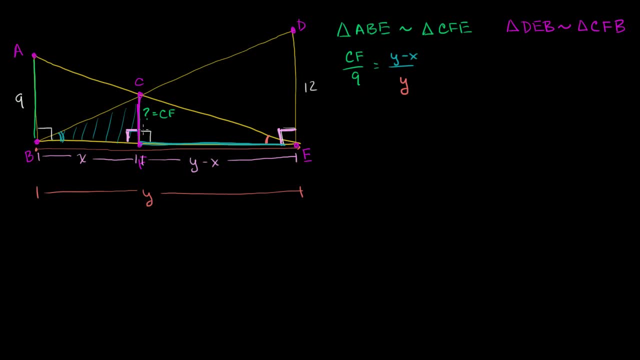 So now we're looking at the triangle CFB, not looking at triangle CFE anymore. So now, when we're looking at this triangle, CF corresponds to DE. So we have CF over. DE is going to be equal to x. It's going to be equal to. let me do that in a different color. 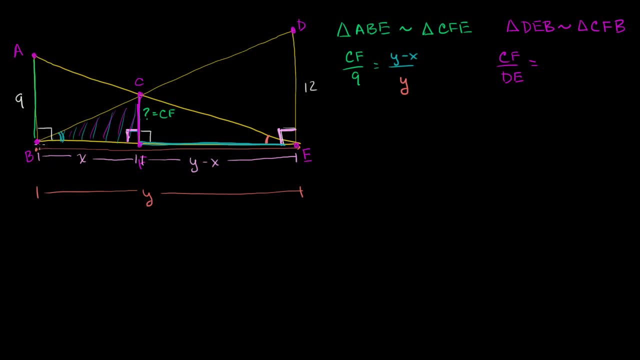 It's going to be equal to: I'm using all my colors. it's going to be equal to x over this entire base, right over here, so this entire BE, which, once again, we know is y, so over y. And now this looks interesting because it looks like we. 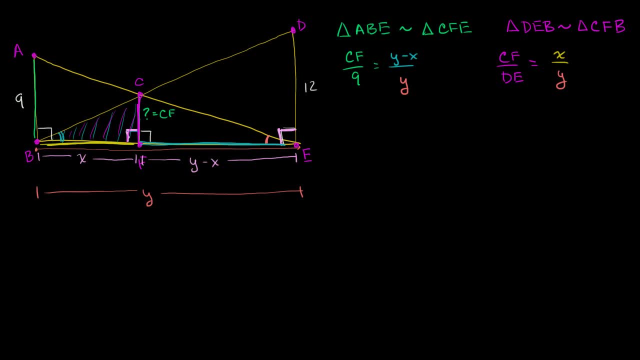 have three unknowns. We have CF. sorry, we know what DE is already. This is 12.. I could have written CF over 12.. The ratio between CF and 12 is going to be the ratio between x and y. So we have three unknowns and only two equations. 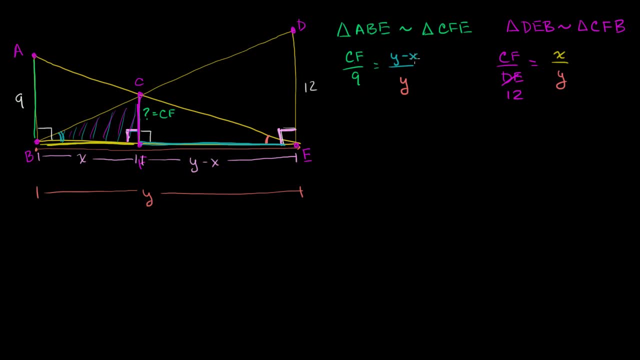 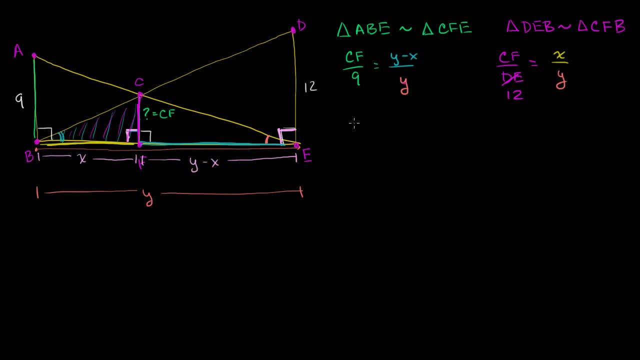 and then we could do a substitution. So that's why this was a little tricky. So this one right here we can rewrite as CF- let me do that same green color. We can rewrite it as: CF over 9 is equal to y. minus x over y is the same thing. 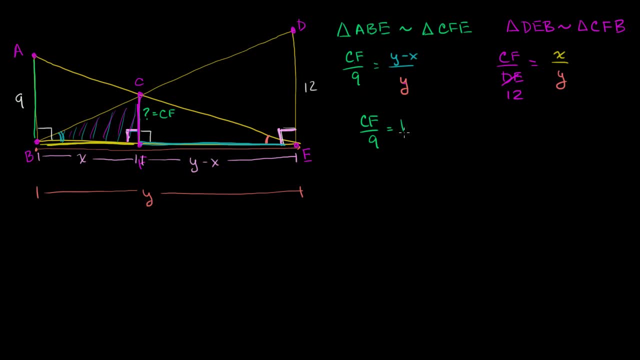 as y over y, minus x over y or 1 minus x over y. All I did is I essentially, I guess you could say, distributed the 1 over y times both of these terms, So y over y, minus x over y, or 1 minus x minus y. 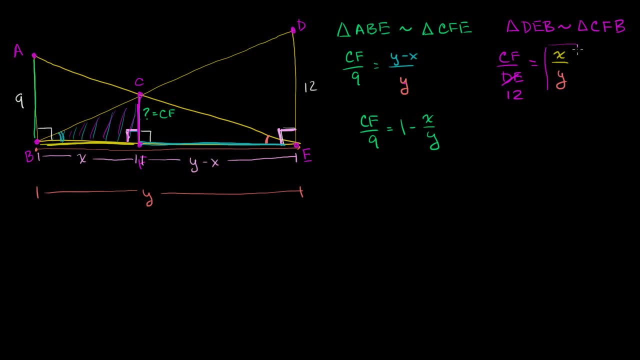 And this is useful because we already know what x over y is equal to. Sorry, We know that x over y is equal to CF over 12. So this right over here I can replace with this CF over 12.. So then we get. this is the home stretch here. 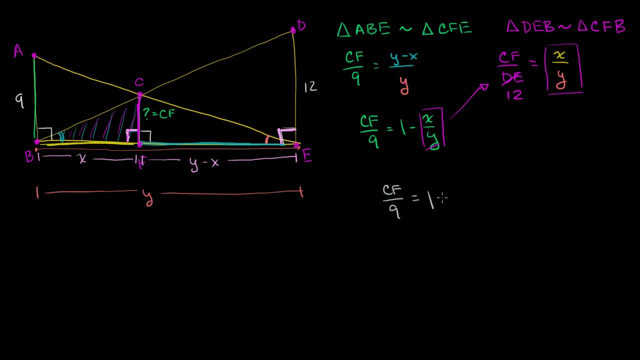 CF, which is what we care about. CF over 9, is equal to 1 minus CF over 12.. And now we have one equation with one unknown and we should be able to solve this right over here, So we could add CF over 12 to both sides. 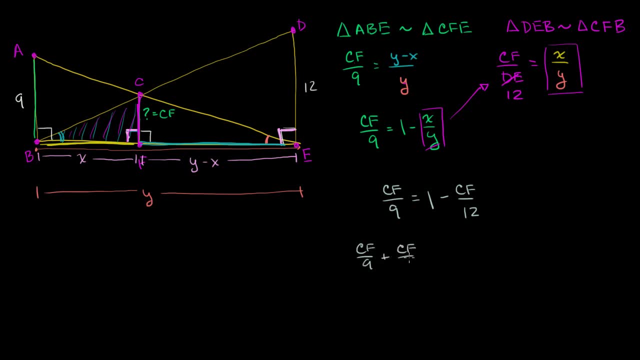 So you have CF over 9 plus CF over 12.. CF over 12 is equal to 1.. We just have to find a common denominator here, and I think 36 will do the trick. So 9 times 4 is 36.. 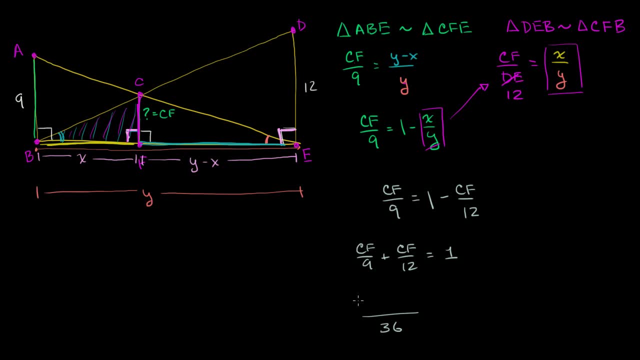 So if you have to multiply 9 times 4, you have to multiply CF times 4.. So you have 4CF. 4CF over 36 is the same thing as CF over 9.. And then plus CF over 12 is the same thing as 3CF over 36.. 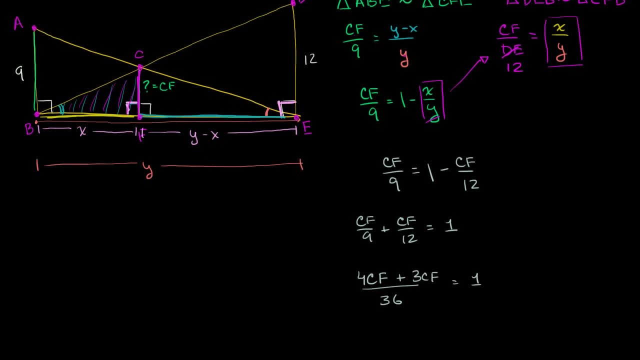 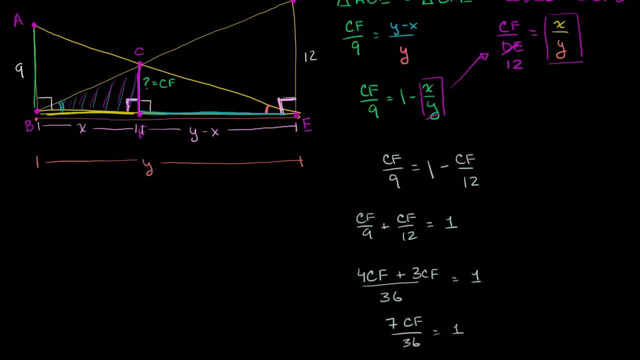 And this is going to be equal to 1.. And then we are left with 4CF plus 3CF is 7. CF over 36 is equal to 1.. And then to solve for CF, we can multiply both sides times the reciprocal of 7 over 36.. 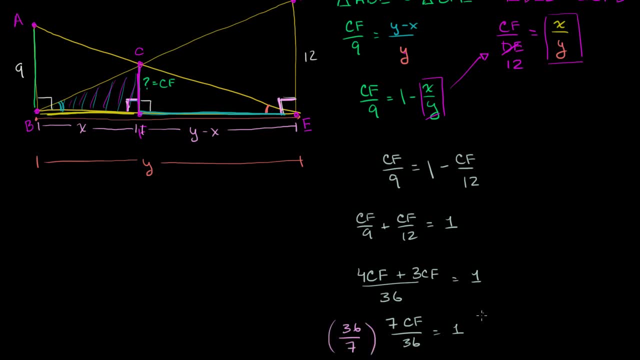 So 36 over 7, multiply both sides, times that 36 over 7.. This side things cancel out And we are left with our final. we get our drum roll. now CF is equal to CF, So all of this stuff cancels out. 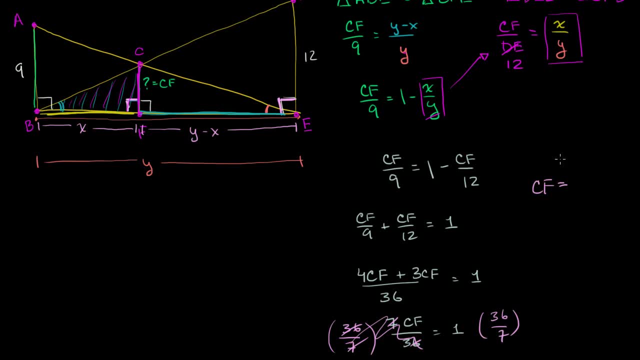 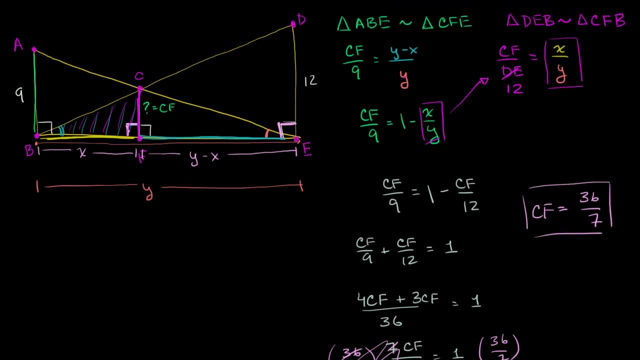 CF is equal to 1 times 36 over 7, or it's just 36 over 7.. And this was a pretty cool problem, Because what it shows you is if you have two things. let's see, this thing is some type of a pole or a stick. 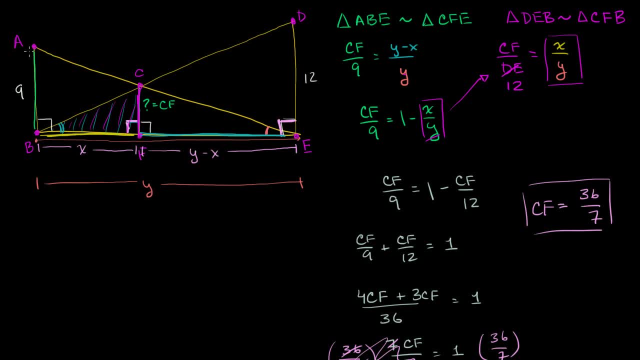 or maybe the wall of a building, or who knows what it is. If this is 9 feet tall or 9 yards tall or 9 meters tall, and this over here, this other one is 12 meters tall or 12 yards or whatever.